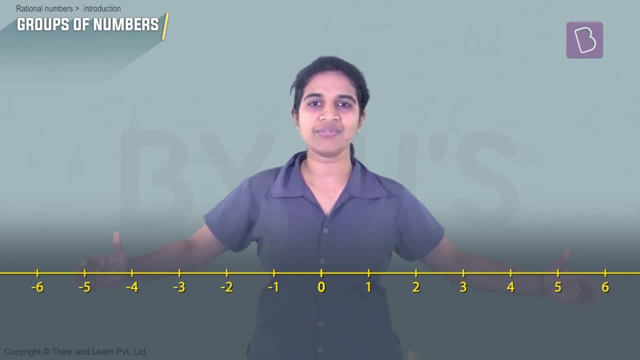 the other side, This entire set of numbers that we now have is called as integral. So we have a set of integers, right, Represented by i. again an infinite set, right? So okay, do we now have all the numbers possible? Seems like a lot, right, But not really. Let's zoom. 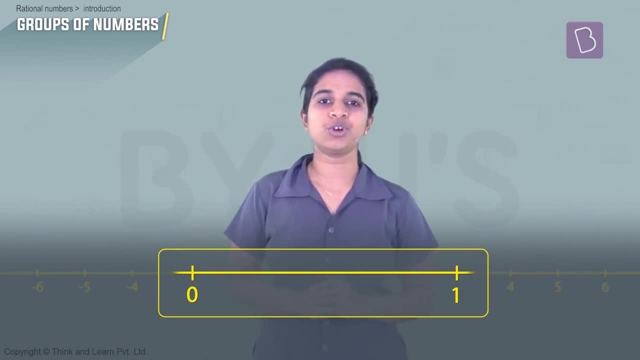 into a section of the number line to see, Let's say, we zoom in to 0 to 1.. Can we have more numbers here? This is one unit, right? This is one unit. Can we divide it into smaller units, is the question. If we can, then we would have numbers in between, right? So? 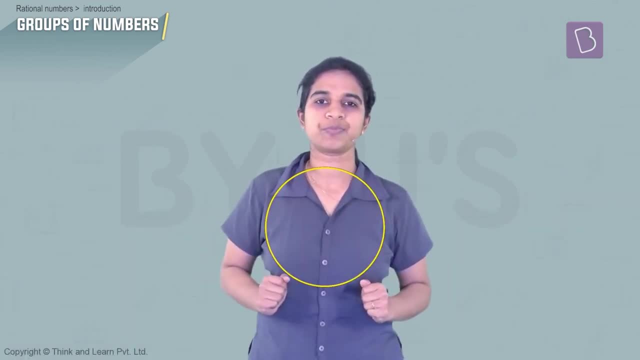 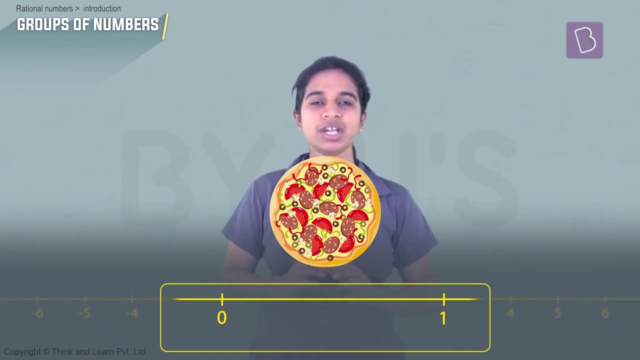 instead of a section. let's imagine it to be 5. To be something like a pizza. right, Let's imagine this to be a pizza. Let's move the line down. Let's have a pizza instead of the number. right Now, can we divide this Essentially? 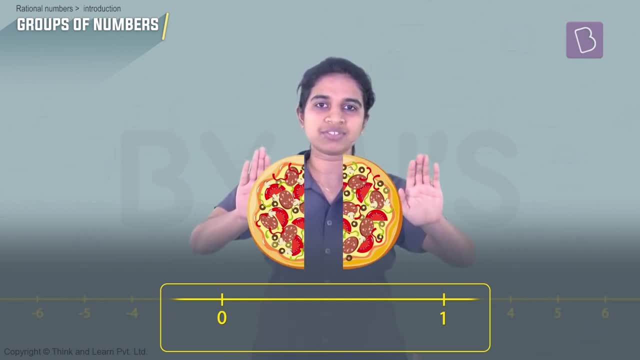 we want to divide this unit. right, This is one unit. We can divide it into two halves, like this, So between 0 and 1, there is one point which is the half correct. Now, if we take this half, you can further divide it into two quarters. You can further divide. 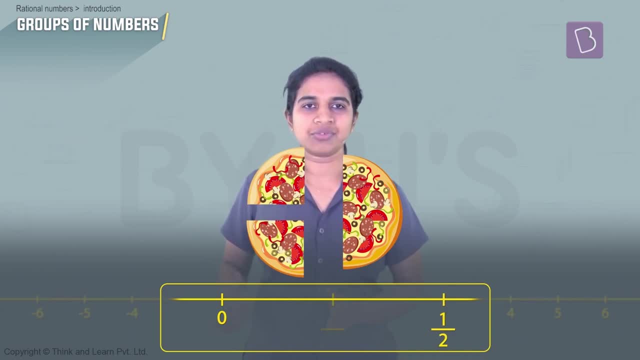 it into two quarters. What does that tell you? Between this half, there is a point which is the quarter right. Similarly, this quarter, you can further have a point 1, 8.. This 1, 8, you can have. 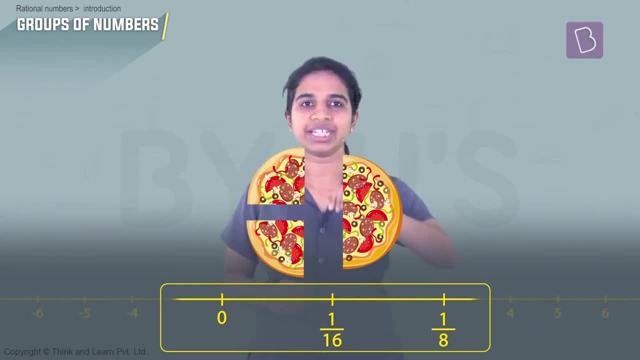 a point: 1, 16th and so on. right, We can keep going, We can keep slicing it into smaller and smaller pieces and we can keep dividing our number line, right. So what does that tell us? That integers are not enough to represent all possible numbers. there are, In fact, between: 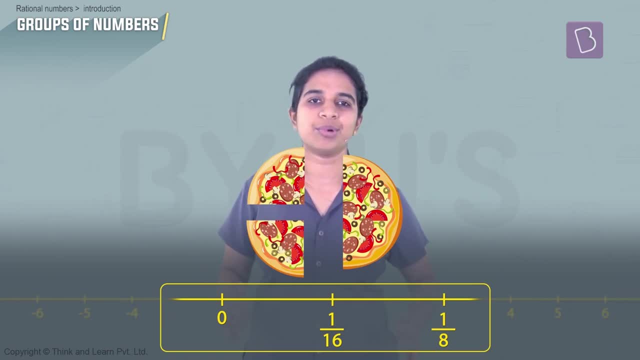 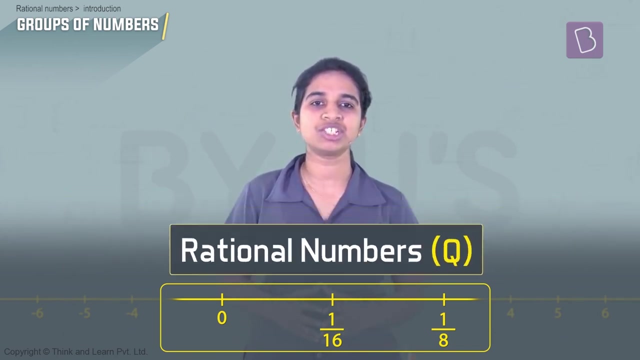 every two integers there are another infinite set of numbers. right, We were able to divide it infinitely. right, going on and on right. so between any two integers, there are again an infinite set of numbers. now, these numbers that we just got are called as rational numbers. right, rational numbers, the. 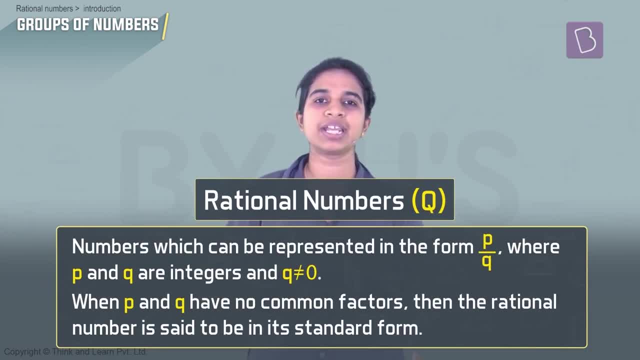 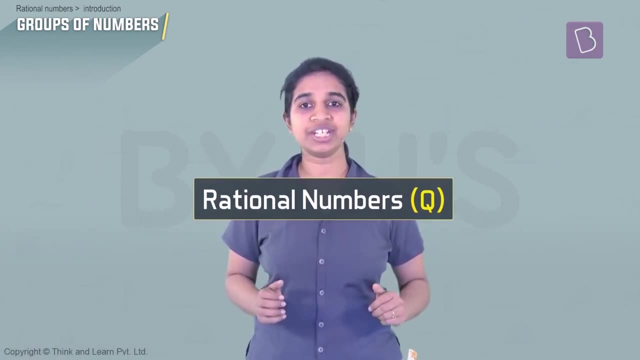 definition for these is nothing but any number that can be represented as p by q, right p by q, where p and q are integers. q is not zero and p and q don't have any common factors, right? so that is essentially what a rational number is, and actually even all the integers are rational.